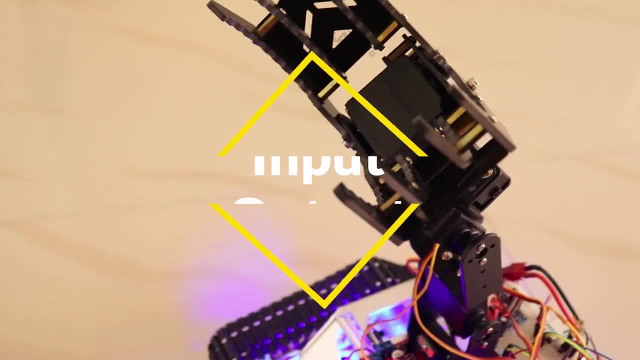 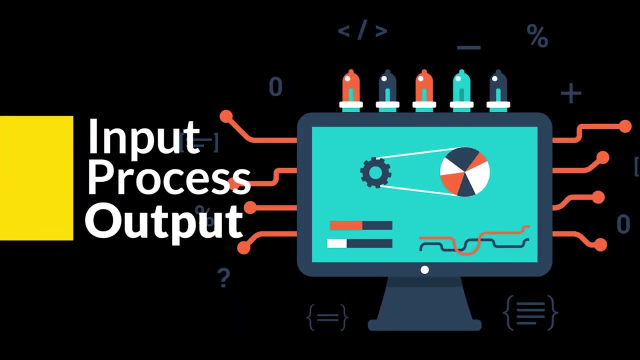 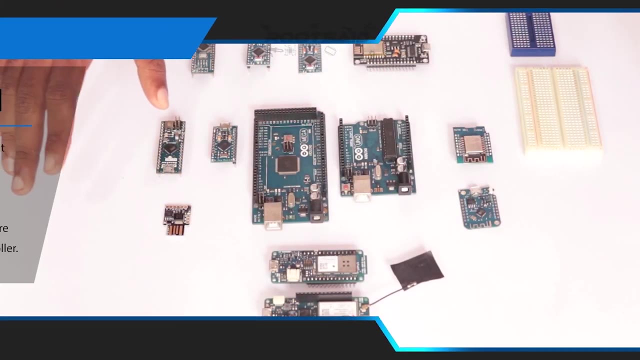 can gather information from the environment, and outputs are devices like motors, LCD displays, which can give us an output. Usually, what we do is we gather input from the sensors, process it using logic circuits and get the response from output units. It's in the processing stage where we use Arduino boards. 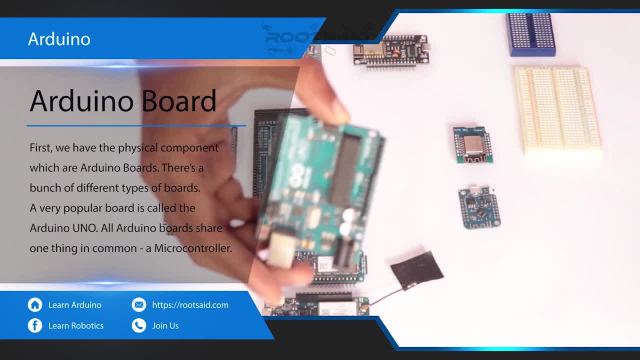 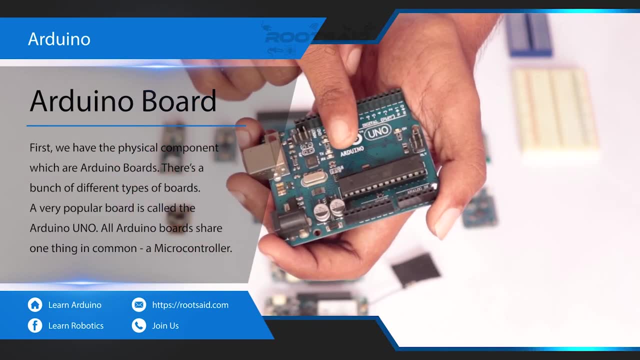 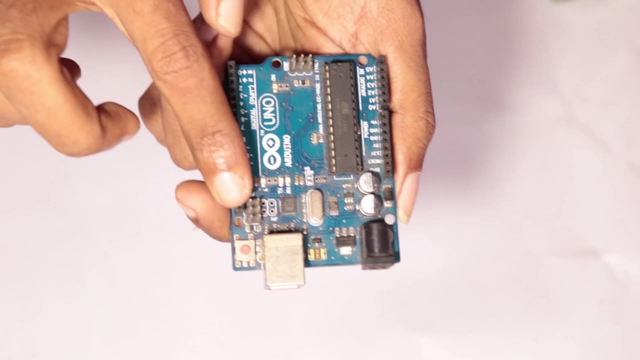 that contain microcontroller. This is a typical Arduino board. Its name is Arduino Uno. You might be familiar with this board if you are into DIY electronics and hobby projects. Now look at this board closely. You should be able to see black holes on either side of the board. These are known. 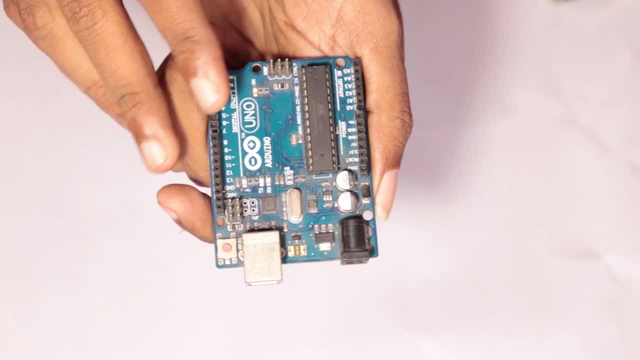 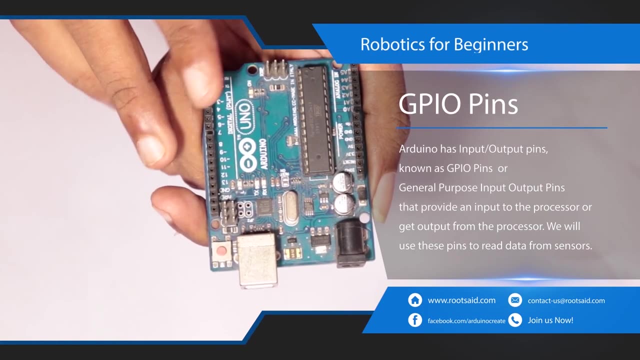 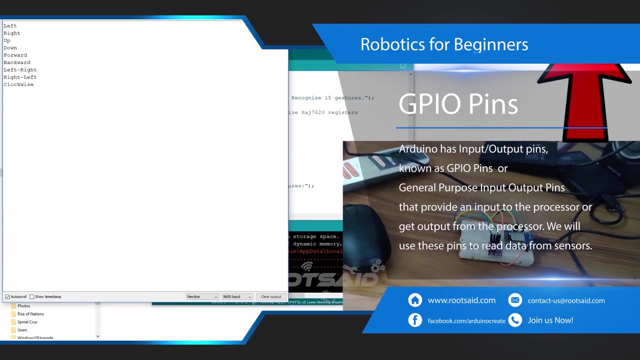 as microcontroller boards. These headers are connected to GPIO pins of the microcontroller internally. GPIO stands for general purpose input output. Using these headers, you will be able to connect various devices like sensors, to the microcontroller via the GPIO pins, without soldering That is. using these headers, you should be able to pass on information from. 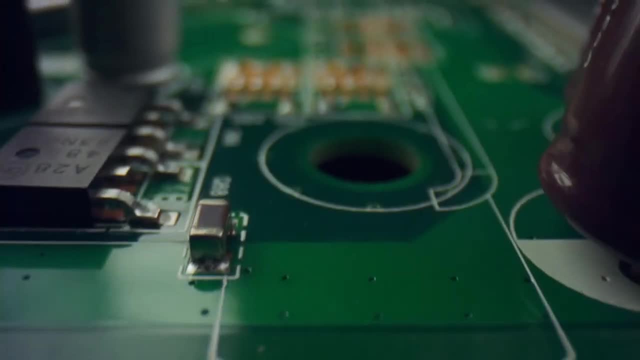 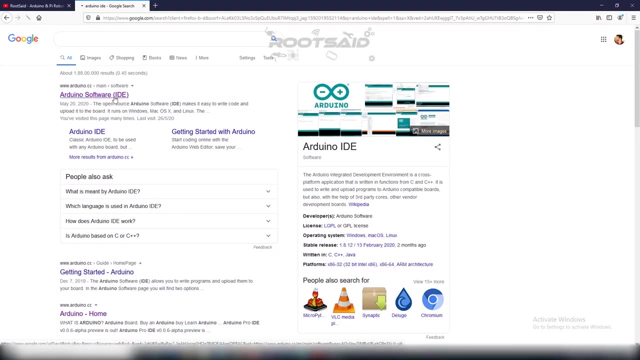 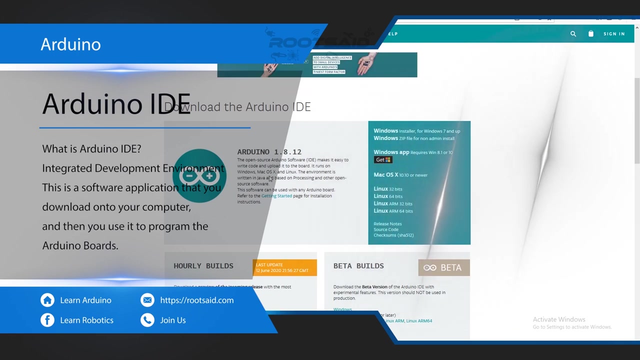 sensors to the microcontroller, process it and pass the process information from microcontroller to the output devices. For starting programming, the first thing you need is Arduino IDE. IDE stands for Integrated Development Environment. It is a free software. If you want to download it, I will leave the link. 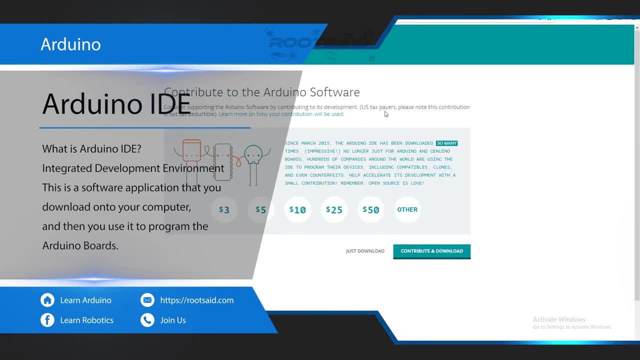 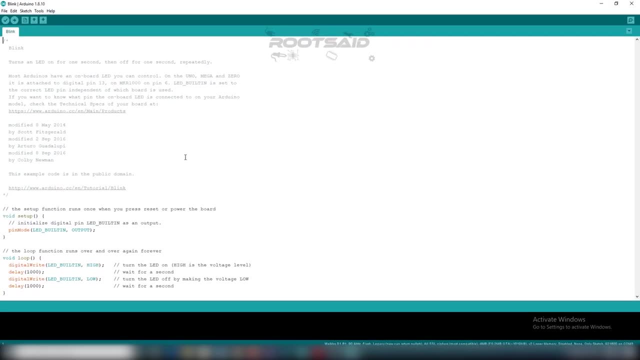 in the description. Arduino IDE is kind of like a lightweight text editor. This text editor is where we write the code for our project, compile it and upload it to our board. This code that we write inside Arduino IDE is known as Arduino IDE. This code is used to write code for our project, compile it and upload it to our board. This code that we write inside Arduino IDE is known as Arduino IDE. 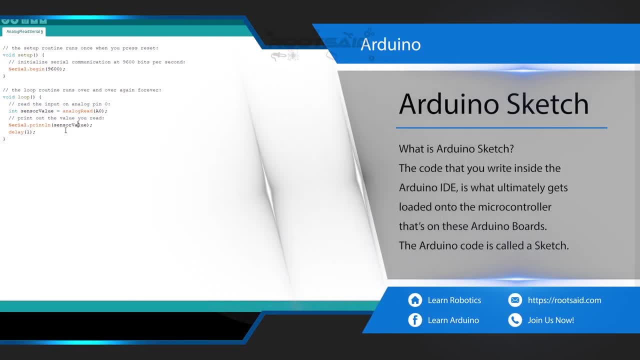 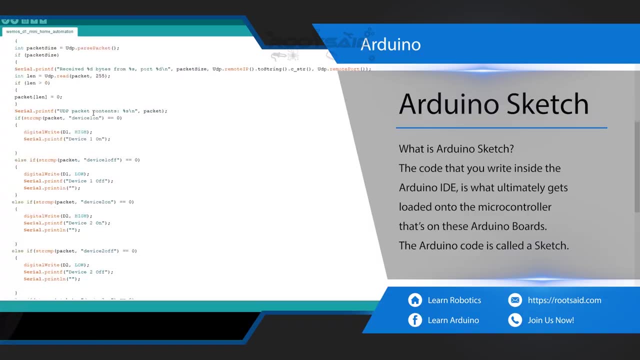 Arduino sketch. It is also very easy to code on Arduino. The language is like a derivative of C++ and is very similar to it. The code is first compiled to a language which is readable by machines and is then uploaded to the board. So that's all the basics you need. 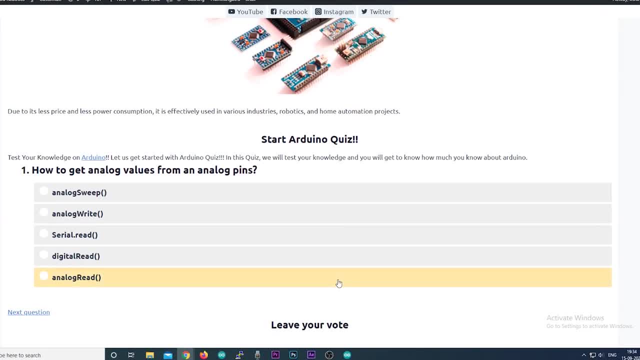 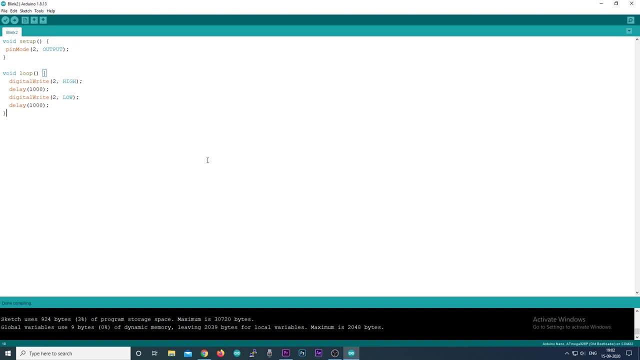 We will now start coding. After this, make sure you attend this quiz and test your knowledge on Arduino, And I think it will be better if I explain with the help of this example. Now, take a look at this code. This is the code for blinking an LED. It looks so simple. right, Because it is simple. Now what do? 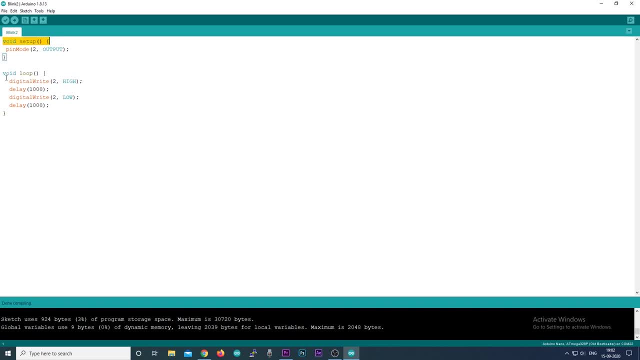 you see, in this code There are mainly two blocks: right Void setup and void loop. You will see these two blocks in all Arduino codes. The first block is void setup. This function will be executed first when the board is first powered on, And this function will be executed only once When the board 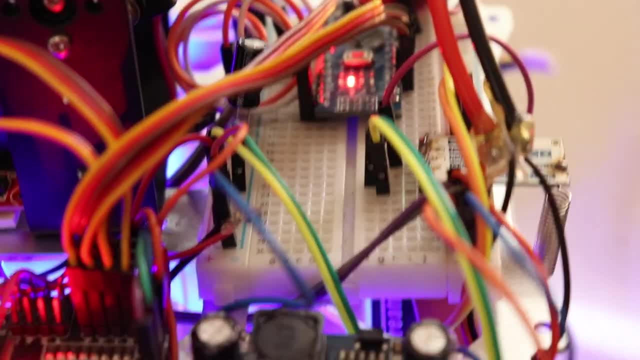 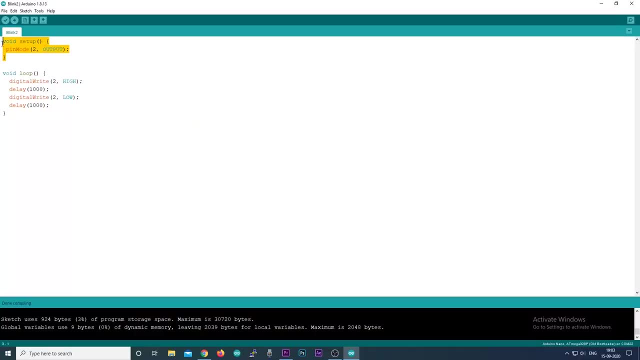 is first powered on. what happens is this function will be run first and prepare the board for running the main commands, which is written inside the loop function, And due to this reason, this block is known as preparation block. As you can see in this example, there is only one line in this setup. 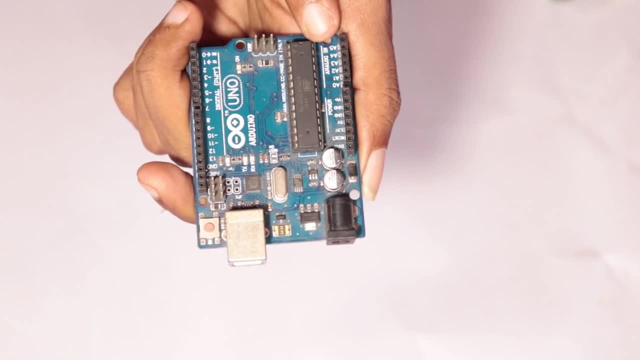 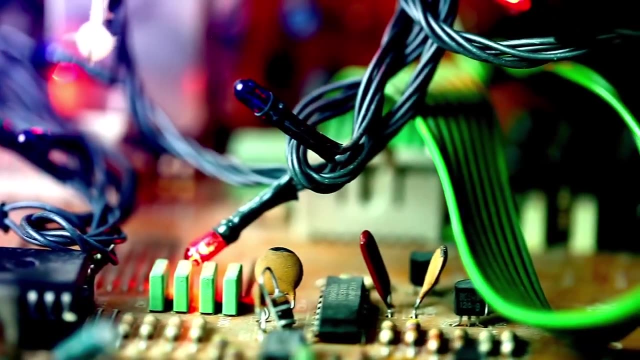 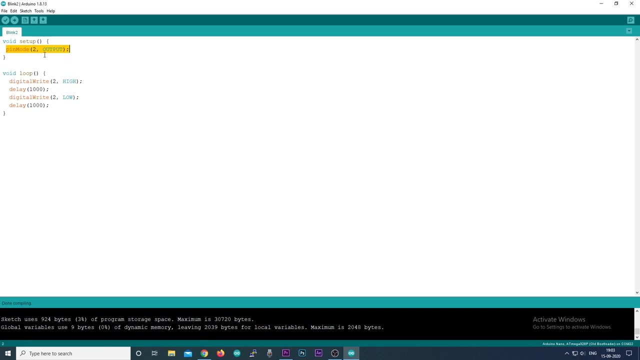 function. Just a minute ago I told you there are numbers for each pin. For this example, LED is connected to pin 2 of this Arduino board. LED is an output device, right? So we are declaring pin 2, where we connect the LED, as an output pin. That's all we need inside the setup function. 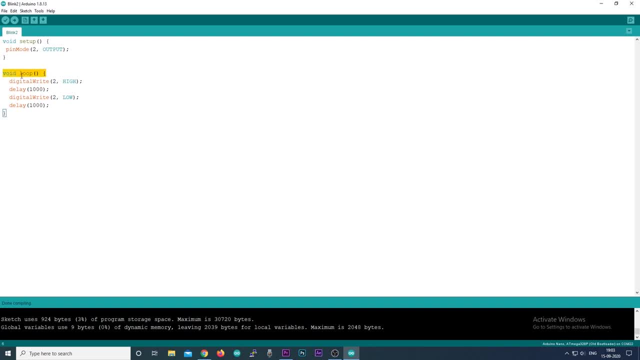 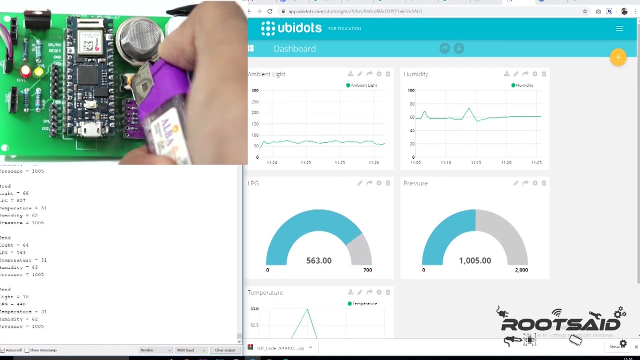 Next we have loop function From the name itself. you must have got the idea right. All the codes inside this function will be repeated again and again, So this block is known as the execution block. All the codes that is required for continuous operation of Arduino boards like. 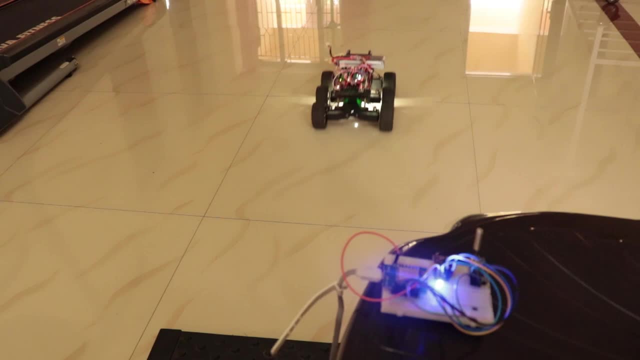 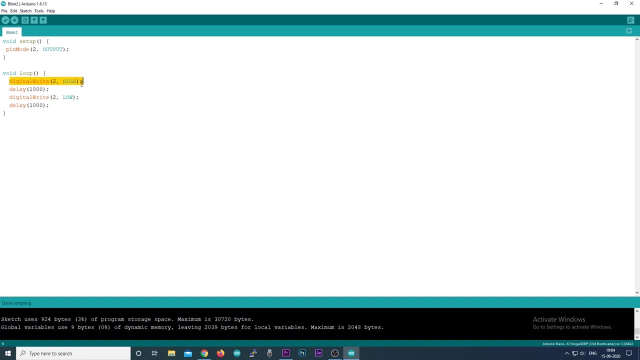 collecting input from sensors, processing it. all these segments are written inside this block. Here you can see 4 lines of code. The first line is digital write to high. This is for declaring the value of the digital output, pin 2 to high. That means it will change the voltage of pin 2. 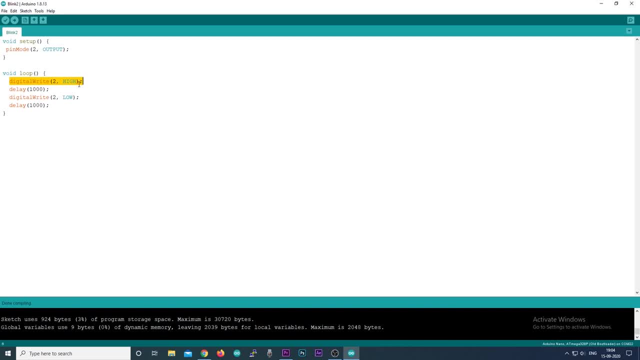 to 5 volt. Now the LED is turned on. We want to keep this on for 1 second. So in the next line we write: delay 1000.. This is not 1000 seconds. alright, It's 1000 milliseconds. 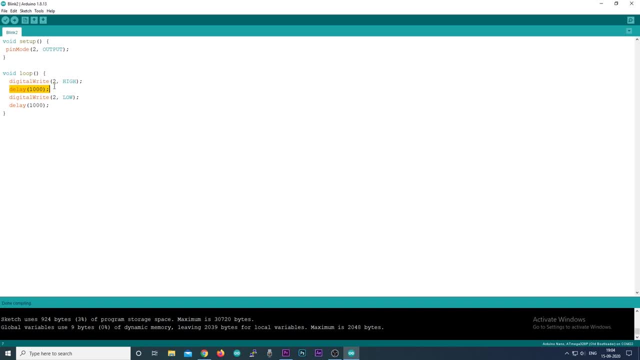 So it will wait for 1 second before executing the next line. Digital write to low. That is exact opposite of the first line and it will change the state of pin 2 to low, That is, 0 volt, Which will turn off the LED. Now we need this LED off for 1 second, So we go for the 4th line.